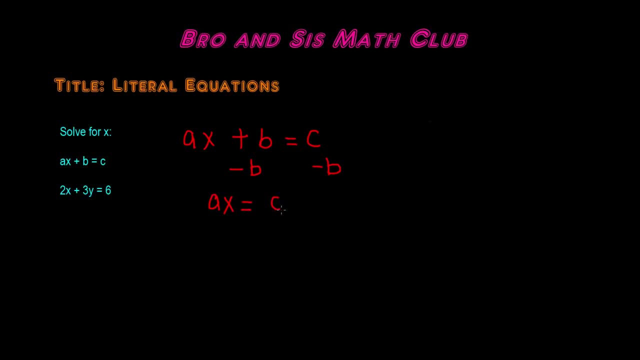 And we're left with: ax is equal to c minus b, Because the positive b and negative b are equal, So negative b cancel each other out. So now we have: ax is equal to c minus b. Now we have to get rid of the a. 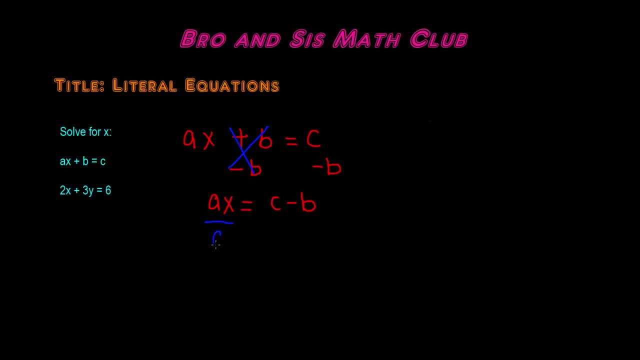 a is being multiplied to x, So we have to divide by a, Because the opposite of multiplication is division. So a and a cancel each other out And we're left with x is equal to c minus b over a, And that's it. 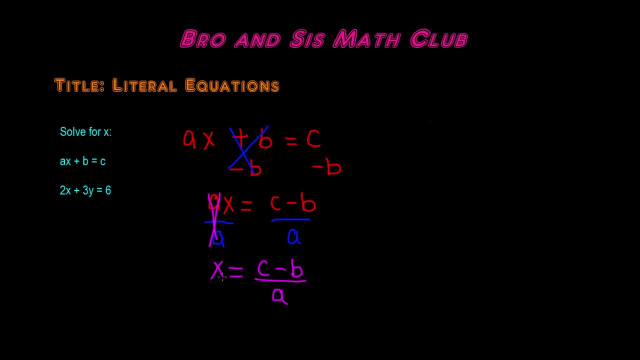 So that's the solution to the literal equation. So, as you can see, we're not trying to find the value of x, We're just trying to isolate it. So x is equal to c minus b over a. Alright, Now let's solve the second literal equation. 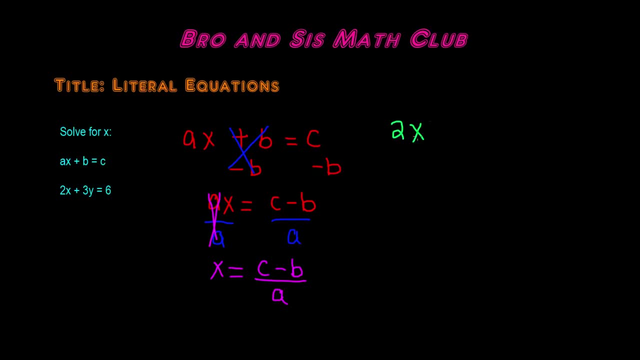 So the second literal equation is: 2x plus 3y is equal to 6.. Remember, we're trying to solve for the variable x, So we need to undo anything that's being done to the variable x, Since 3y is being added to x and 2 is being multiplied to x. 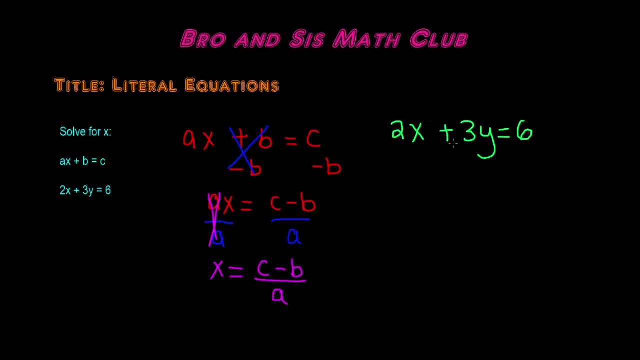 We need to get rid of these. So first, let's get rid of the 3y. Since it's a plus 3y, let's do minus 3y, Because the opposite of addition is subtraction. Remember to do the same thing on both sides. 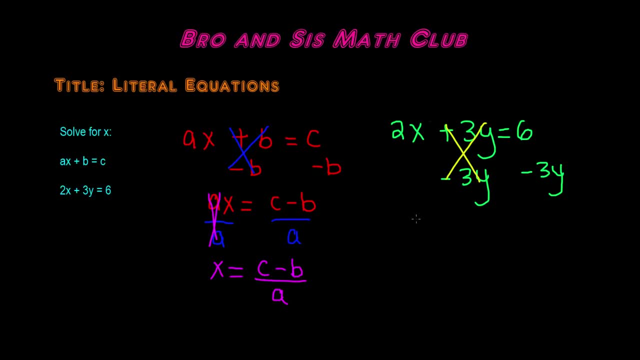 So plus and minus cancel each other out And we're left with: 2x is equal to 6 minus 3y. Next we have to get rid of the 2.. Since it's being multiplied by 2. Let's divide by 2.. 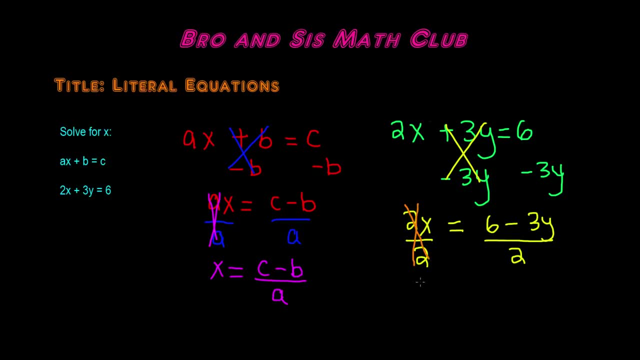 So the 2's cancel each other out And we're left with x is equal to 6 minus 3y over 2.. Or if we simplify, Let's divide 6 by 2 and minus 3y by 2.. 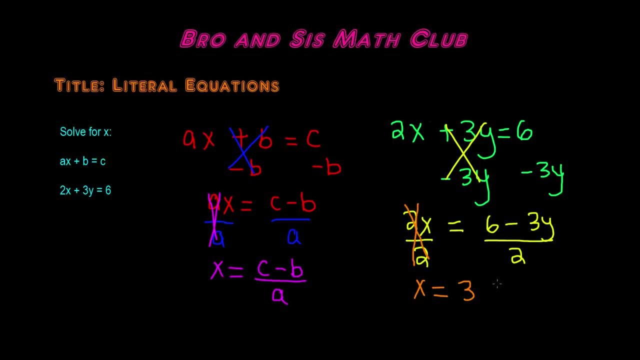 6 by 2 gives us 3.. The minus 3y over 2.. A negative divided by positive is always a negative, And 3 divided by 2 will stay as it is, So it would be 3 over 2.. 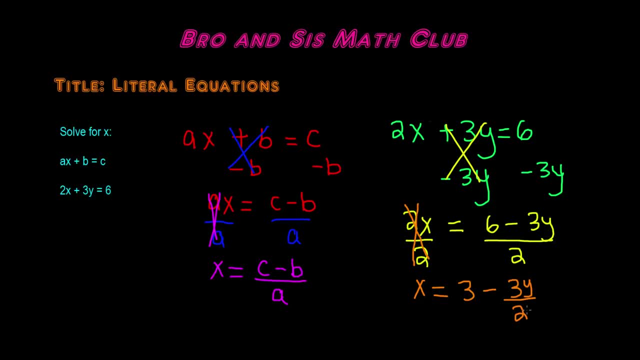 And it's 3y, So 3 minus 3y over 2.. So this is the simplified answer to our literal equation. So this is how you solve literal equations And, as I said, it's really simple Because you're just trying to solve for one variable.